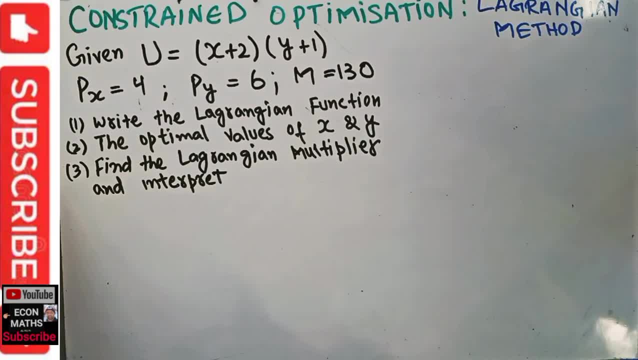 In this video we will solve a question on constrained optimization using Lagrangian method. The question is: given the utility function is: u is equal to x plus 2 times y plus 1, where x and y are the two goods, Price of good x is 4 and price of good y is 6.. Income is 130. 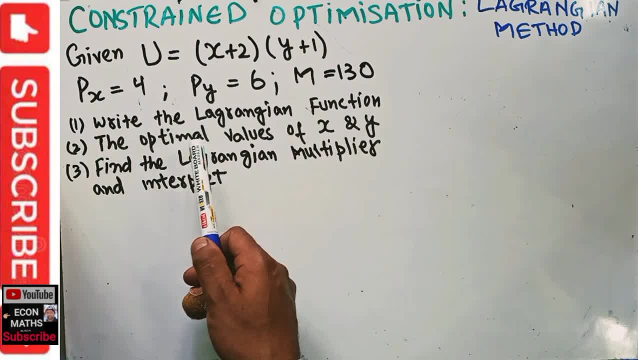 We have to write the Lagrangian function first, Then we need to find the optimal values of good x and y and the Lagrangian multiplier and we need to interpret it. Okay, so let's say we are being given the utility function. u is equal to x plus 2 times y plus 1.. Okay, so we can rewrite it in. 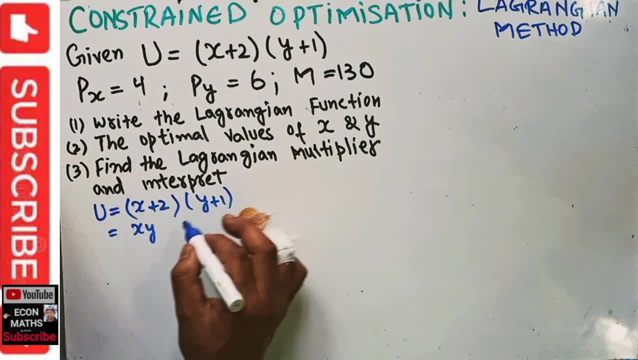 this fashion: x, y, multiplying this x to each of the terms here. So then we have plus x plus 2, y plus 2.. Okay, this is our utility function and we have the budget constraint, that is, price of x times units of good x, plus price of good y times units of good y should. 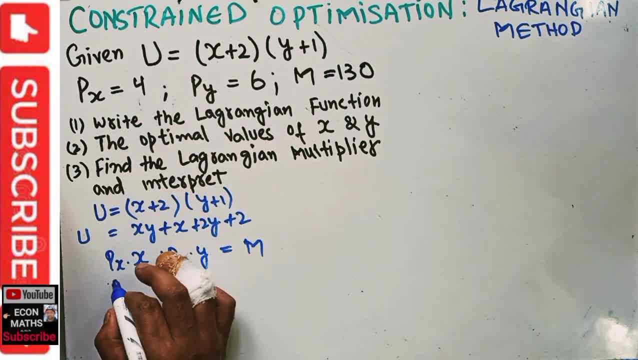 be equal to x plus 2, y plus 2.. Okay, so we can write it in this fashion. So price of good x is 4.. So we can write 4 times x plus price of good y is 6 times y. 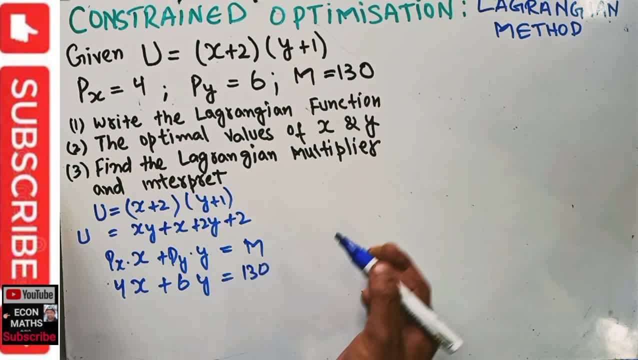 is equal to budget of the consumer is 130.. Our question becomes then: we want to maximize this utility function. u is equal to x, y plus x plus 2, y plus 2.. Okay, subject to the budget constraint, that is, 4 x plus 6, y is equal to 130. 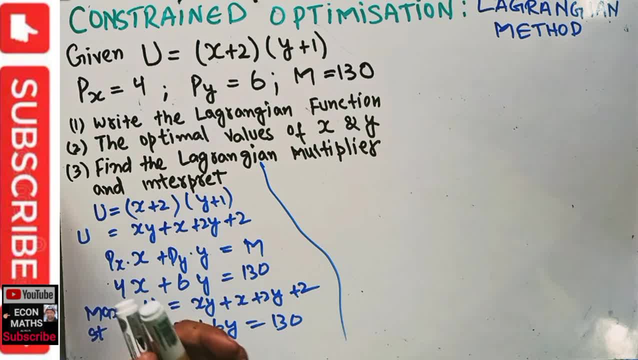 Okay, so this is our question. So what? first we need to find out the language and function. Okay, so language and function can be found by we add this utility function and first we, you know, manipulate this budget function in such a way. If I transpose all the terms to: 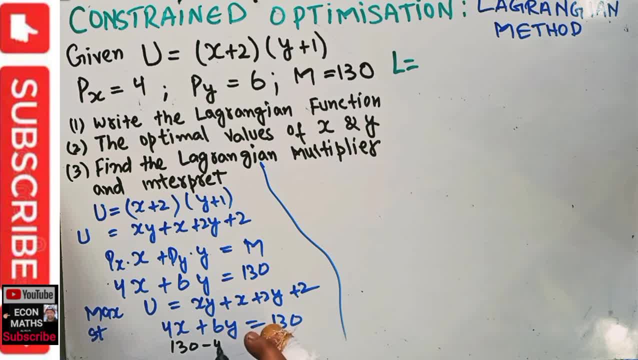 RHS. so it will become 130 minus 4 x minus 6, y is equal to 0.. Okay, so first we said this budget function is equal to 0. Then we multiplied by lambda. Okay, so simple thing is to find out the languages function. 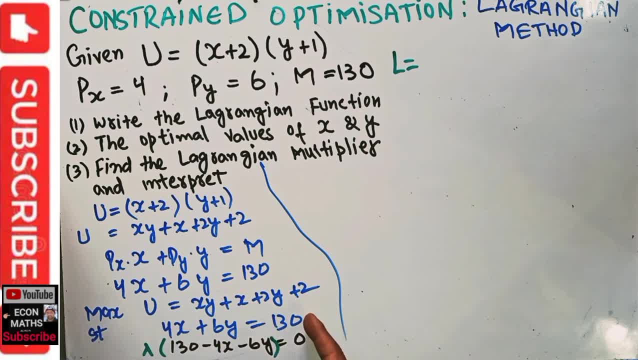 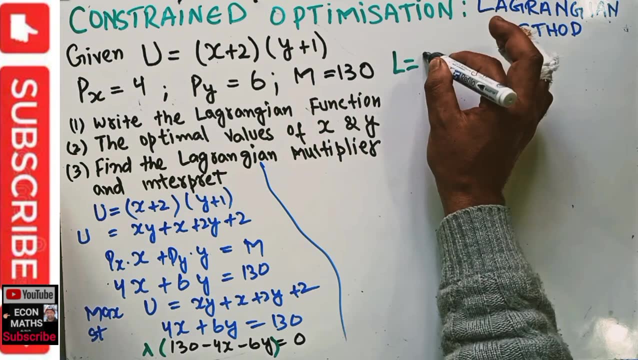 First we need to, you know, manipulate this budget constraint. First we set it equal to 0 and multiply it by lambda, Then our languages function is the given utility function, what we call the objective function, plus this resulting, you know, budget constraint. So it will become 4 x plus 6 y. 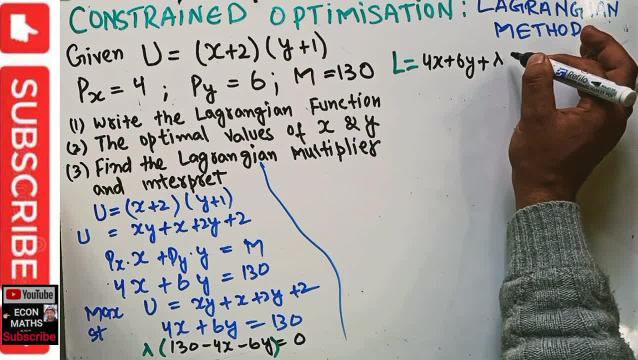 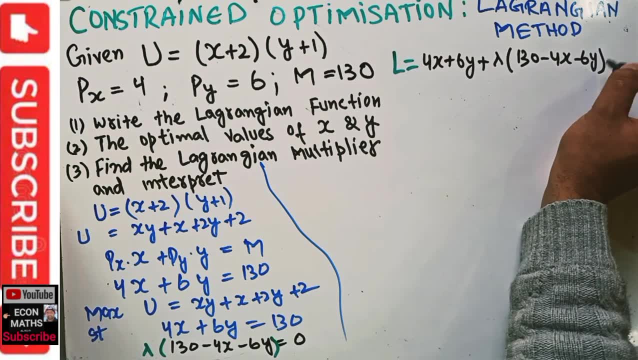 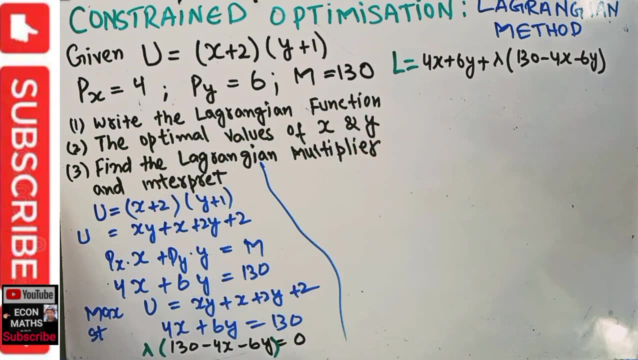 plus this resulting- uh you know uh- budget constraint, that is 130 minus 4x minus 6y. okay, this is our languages function. now the second part tells us to find out the optimal values of good x and y. so we can find out the optimal values of good x and y. simply, part, uh, simply. 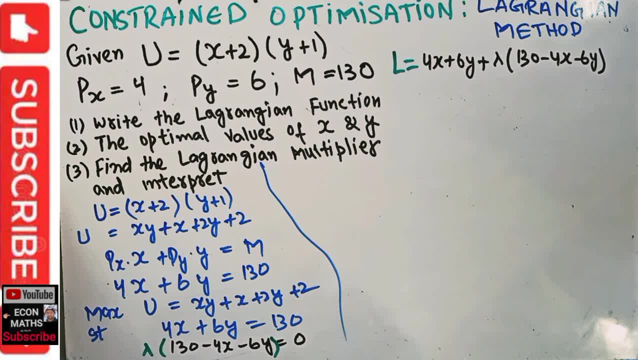 by partially differentiating the given languages function with respect to x, y and lambda and set them equal to 0 simultaneously. that means uh l subscript. x means partially differentiating this languages function with respect x. the derivative of x is 1, so we are left with 4 and derivative of: 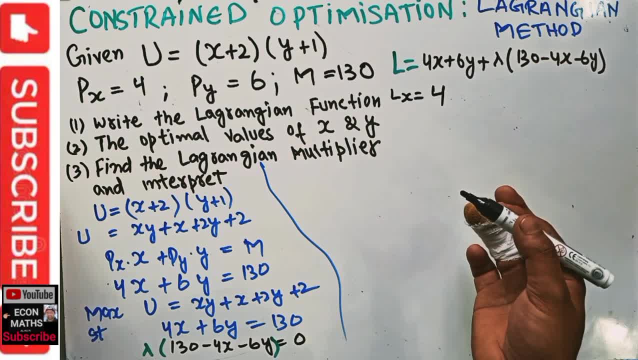 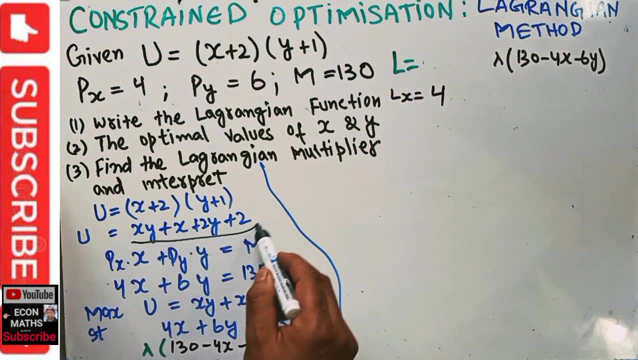 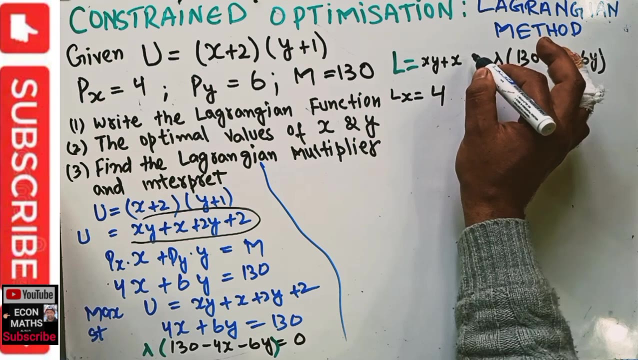 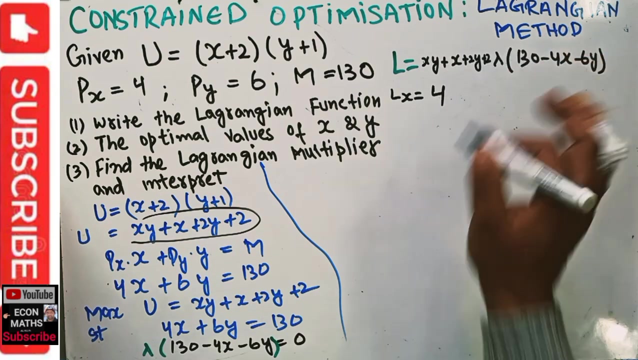 x here is 1, so we are left with minus 4 lambda. okay, so i i guess i have done some mistake here. our languages function is: we have x? y plus x. okay, sorry, uh, this is our uh, you know uh- utility function, that is x? y plus x, x, y uh plus x plus x, x y plus x plus 2, y 2 y plus 2. okay, let me rub this out. 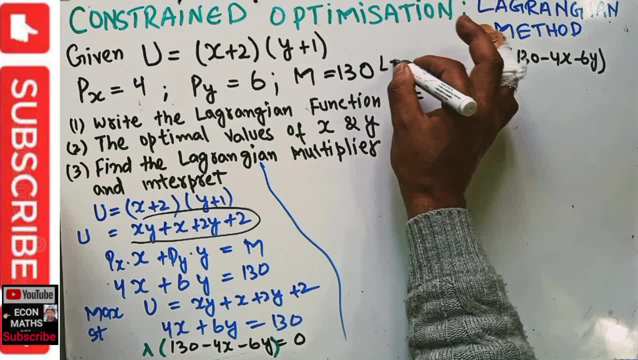 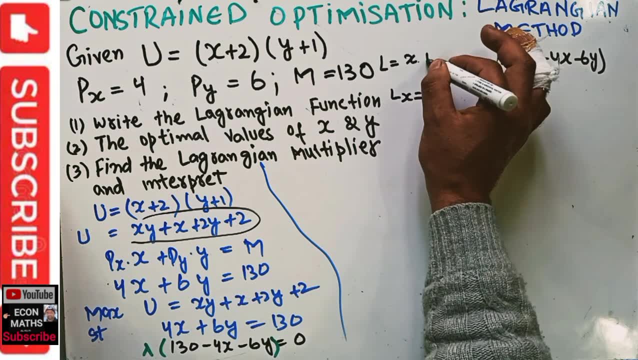 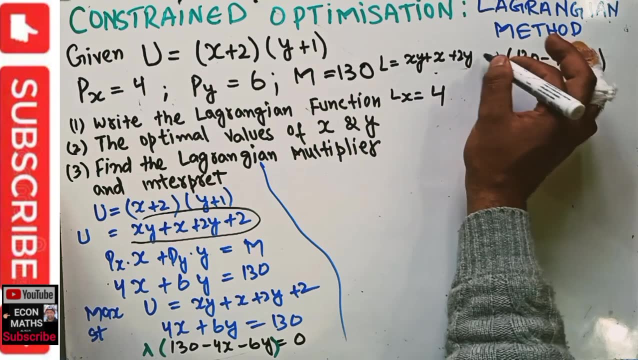 so our l is lagrange's function. is this, uh, the utility function? that is x? y plus x plus 2 y, so x plus. sorry, it is x? y plus x plus 2, y plus 2, okay, plus this resulting constraint. okay, we partially differentiate it. 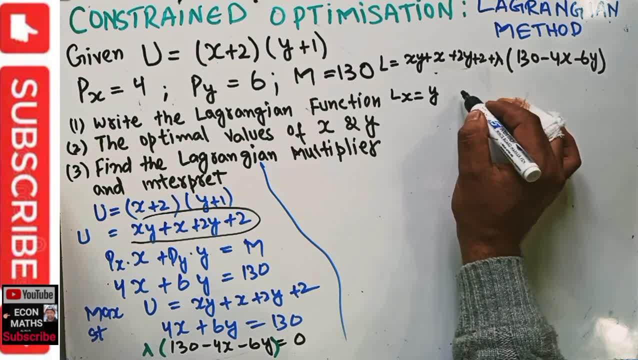 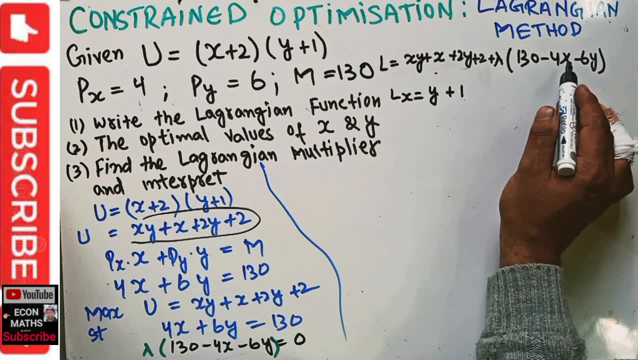 with respect to x, derivative of x is 1, so we are left with y plus. derivative of x is 1, so we are left with 1, and derivative of x here is, you know, 1, so we are left with minus 4 lambda. so we have. 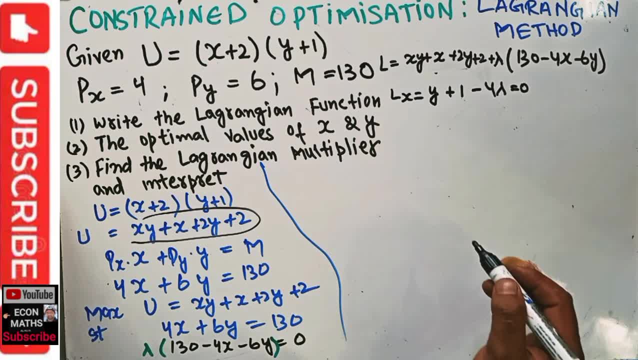 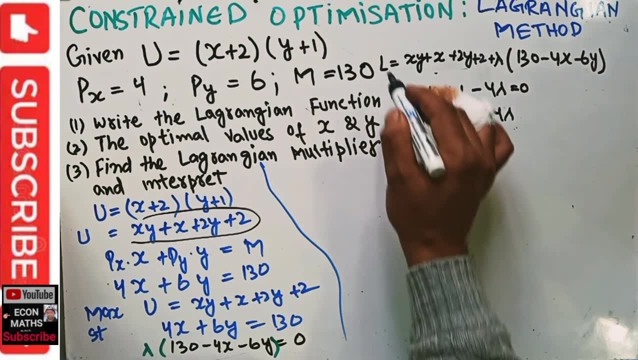 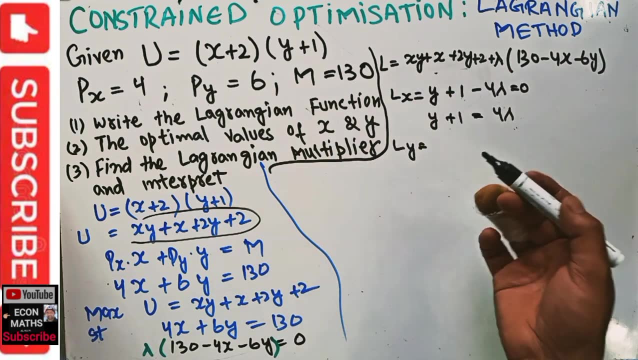 minus 4 lambda, and we set it equal to 0. okay, and we rewrite it in this fashion: y plus 1 is equal to 4 lambda. similarly, uh, what we do? uh, we take the partials with respect to y of the given, uh, rather, of this allegrages function this time. so derivative of y is 1, we are left with x plus. 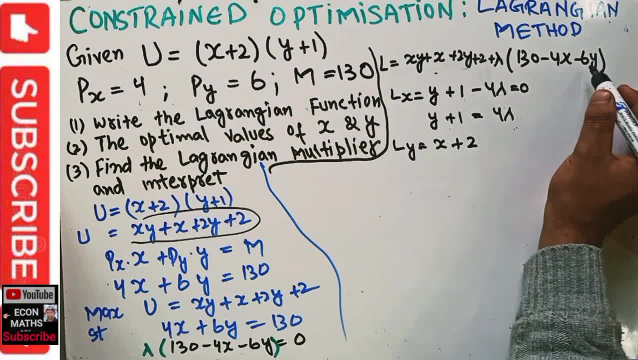 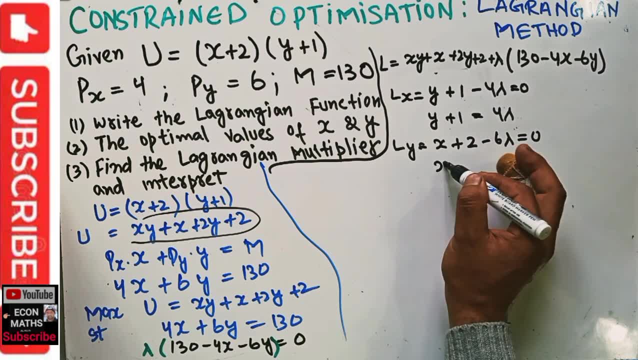 derivative of y is here 1, so we are left with 2. derivative of y is 1, so we are left with minus 6 lambda, minus 6 lambda, and we set it equal to 0. that means x plus 2 is equal to 6, y. 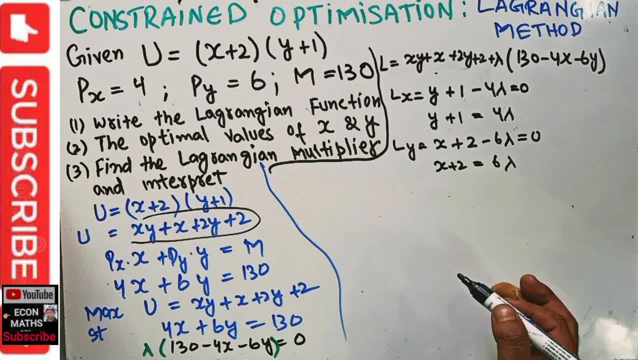 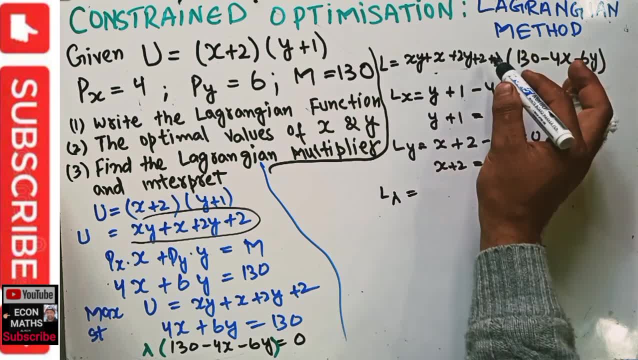 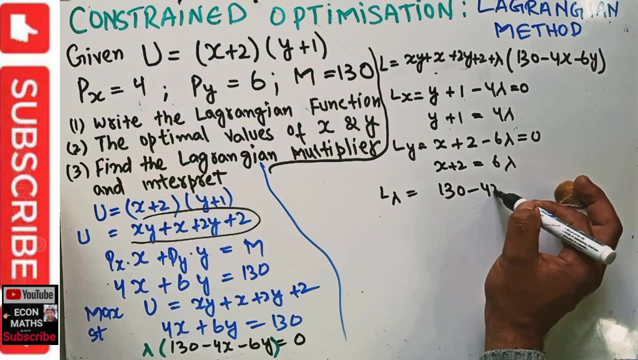 sorry, 6 lambda. then we partially differentiate. uh, this with respect to lambda, that means l of lambda is equal to. so, since no lambda is involved, uh, in the first four terms, derivative of lambda is 1, so we are left with 130 minus 4 x, minus 6 y, okay, and we set it equal to 0. okay, so we have. 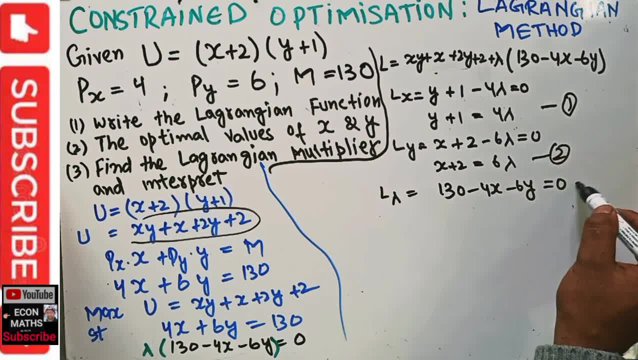 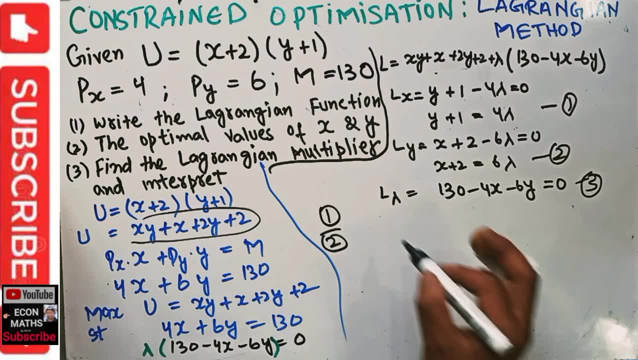 three equations. this is equation first, equation second and equation third. what will we do? we divide equation one by equation second, equation one by equation second. so we have, which implies: y plus 1 divided by x plus 2 is equal to four lambda, four lambda divided by six lambda. lambda lambda gets cancelled, so we have two. 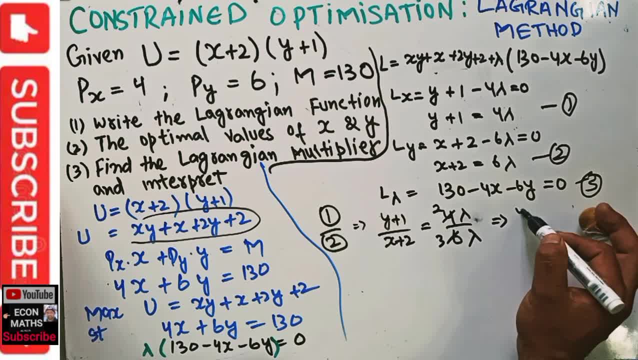 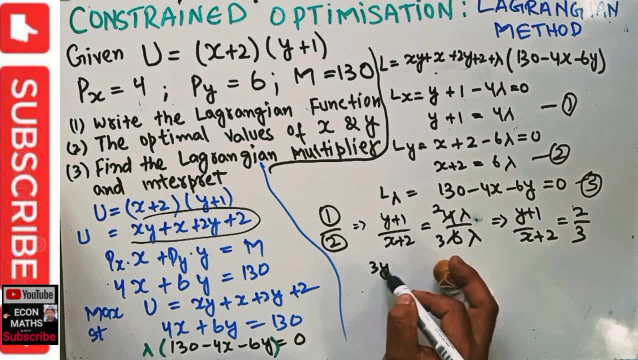 twos are four, two threes are six. so we are left with, which implies y plus 1 divided by x plus 2 is equal to 2 upon 3.. let us solve this So this becomes: 3y plus 1 is equal to 2x plus 2, that gives us, you know, y will be. 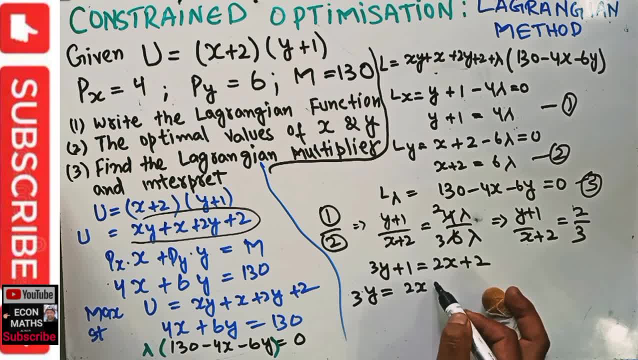 equal to, rather, 3y will be equal to 2x plus 2, sorry, it is here 2x plus 4,. okay, 2x plus 4, so we have 2x plus 4 and transposing this, it will get subtracted. that means: 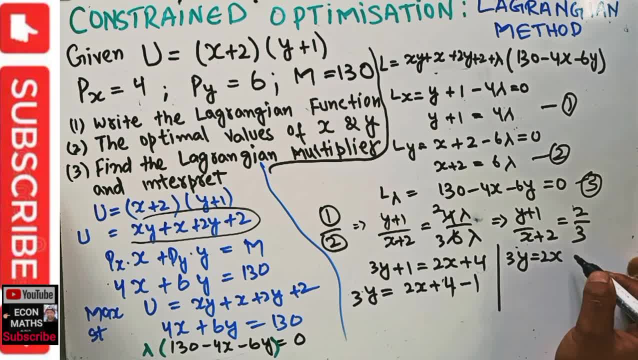 3y is equal to 2x. 2x plus 3, that means let's divide both sides by 3, that gives us y will be equal to 2 upon 3x. am I doing it correctly or not? so 4 minus 1 is 3,. let. 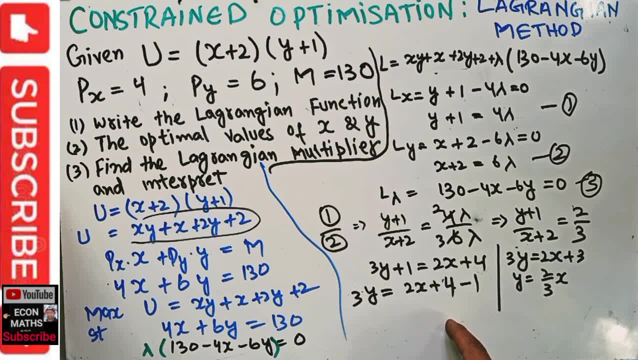 me see here. Okay, I guess I have done some mistake here somewhere. so we have 3y into 1 is 3, so it is here 3,. sorry, I am doing some basic mistakes here. so it is here 3, so this will become 2x. 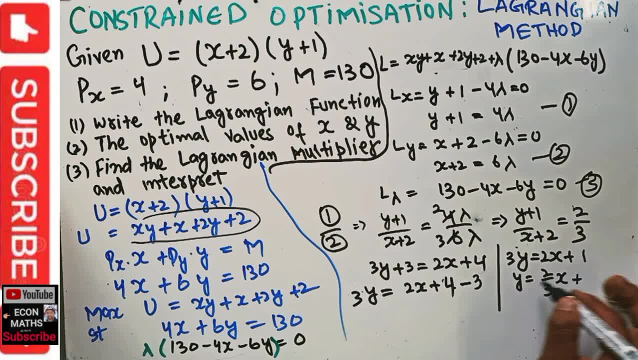 plus 1, okay, so plus. here we have 1 upon 3, now we plug this value of y is equal to this stuff- into the budget constant Or in the third term. okay, so let's plug the value into the into this third equation. 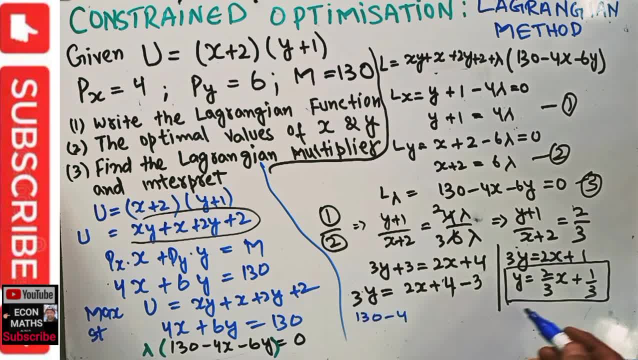 so we will get 130 minus 4x. then we have minus 6, the value of y is 2 upon 3x plus 1 upon 3, okay, and it is equal to 0, so we have 130 minus 4x. here 3 ones are 3 twos. 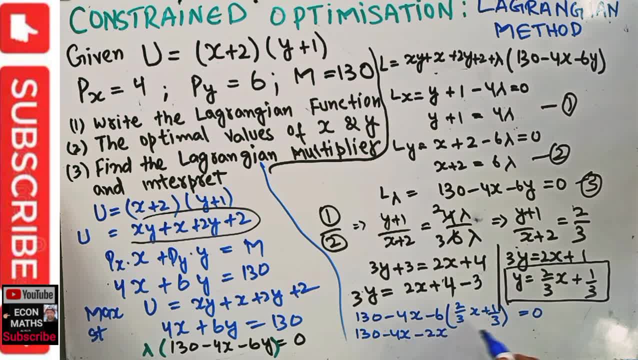 are 6, so we are left with this Minus twice x again. 3 ones are 3, twos are 6, we will be left with minus 2, and we set it equal to 0.. When solving this, this is minus 4x and minus 2x is minus 6x again. I am doing some basic. 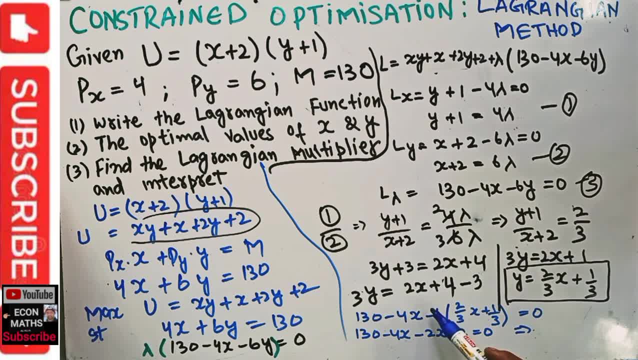 mistakes here. so 3 ones are 3, 3 twos are 6, so 2 twos are 4, it is here 4, okay, so minus 4 minus 4 is minus. sorry, when I transpose it it will become 8.. 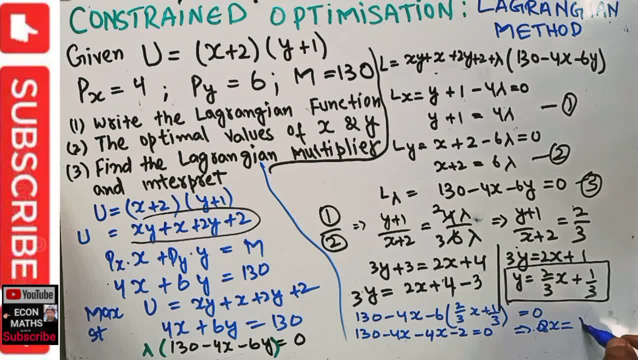 8x is equal to 130. minus 2 is 128, okay, dividing both sides of the x, we will get the value of x equal to 128. divided by 8 will be equal to 8 ones are, so we get the optimal value. 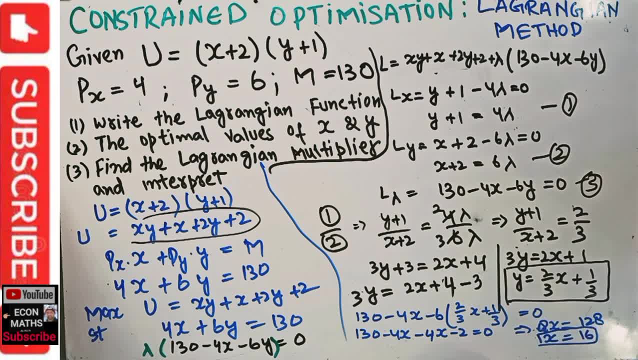 of you know, optimal value of good x is 16.. To find out the optimal value of good y, so simply plug. x is equal to 16 in this equation that gives us, y will be equal to 2 upon 3.. 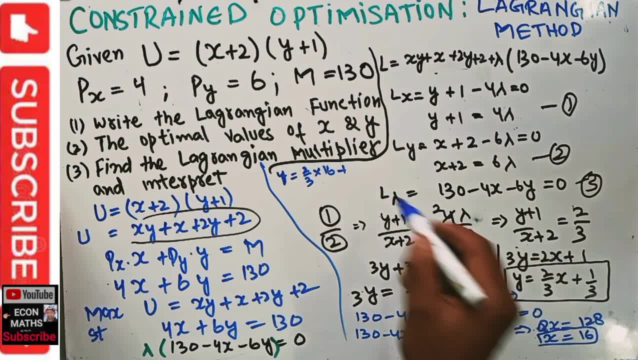 Times 16 plus 1 upon 3, solving this it will give us the value of, you know, y equal to 11, okay, so we got the optimal values of good x and y. Now the third part tells us to find out the Lagrange's multiplier. 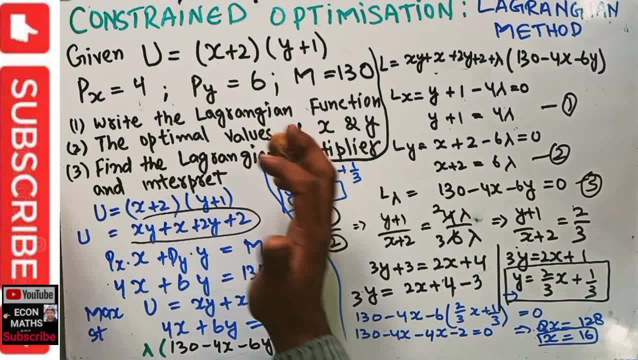 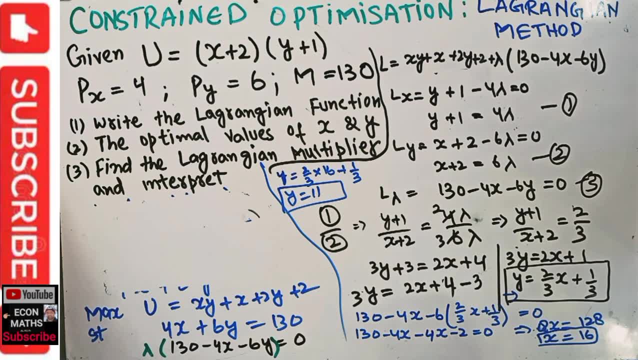 For that. let me rub something here. okay, let me rub this out To find out the Lagrange's multiplier. what will we do? We simply plug the optimal values of x and y. This is an equation first, our equation second. let us solve it for our equation first. 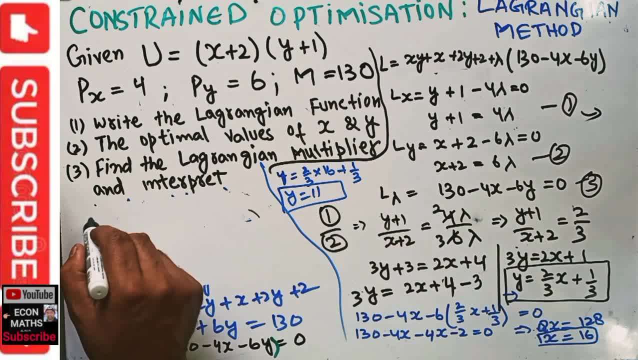 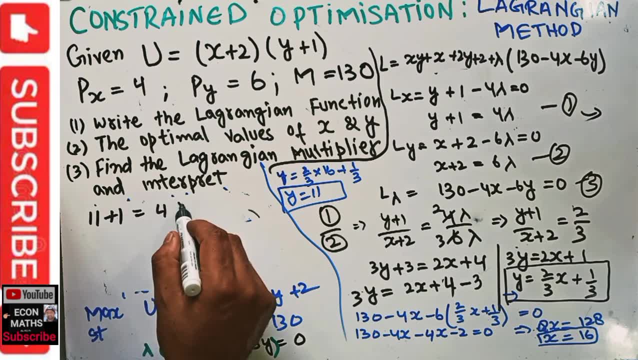 So y in place of y we write the optimal value, which is: 11 plus 1 is equal to 4 lambda. so 4 lambda 11 plus 1 is 12, is equal to 4 lambda. that gives us the Lagrange's multiplier. 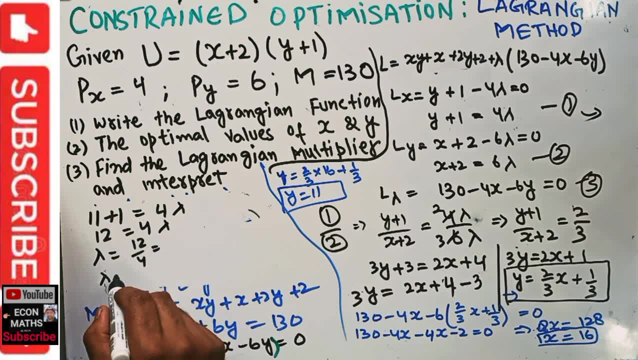 equal to 12 upon 4, which gives us Lagrange's multiplier equal to 3, and to interpret it, it simply tells us: Okay, How does the utility changes when there is change in the constant constant of the budget constraint? okay, simple thing. 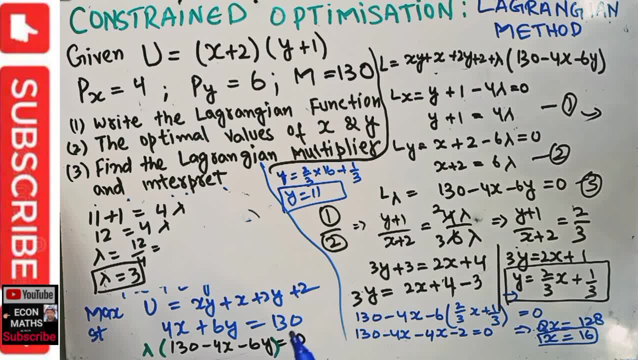 How much utility will change if the constant of the constraint changes. So what is the constant of our constraint? It is income here. okay, So it simply tells us we got budget. rather, this Lagrange's multiplier is 3, it simply 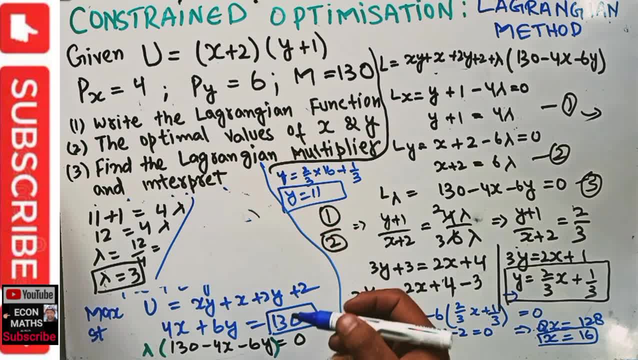 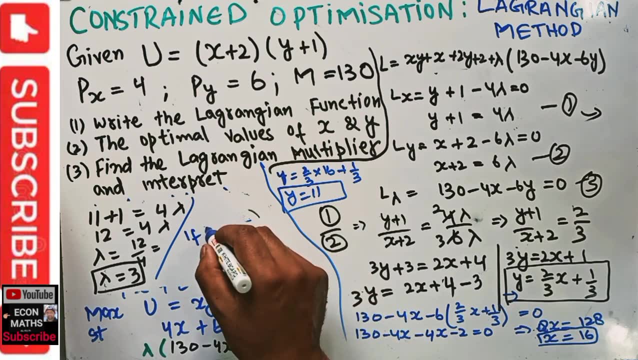 tells us how much utility Utility will change if there is change in the constant of the constraint. so the constant of the constraint is here 30, so it simply tells us, if you know income increases by 1 unit, okay, utility utility will increase by 3 units, okay.